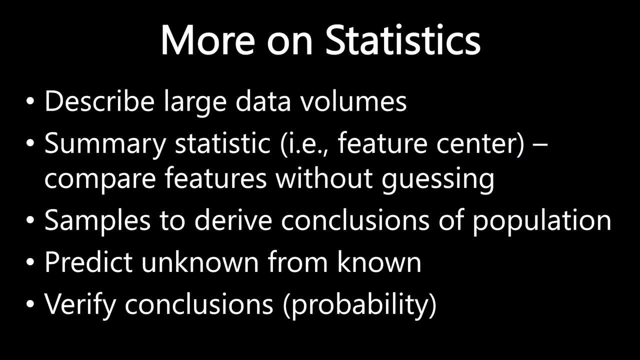 Like traditional statistics, spatial statistics are also interested in describing large volumes of data, such as the center of features and the center of values. These data Icelandic researchers use run samples to derive conclusions from populations, attempting to predict the unknown from the known. 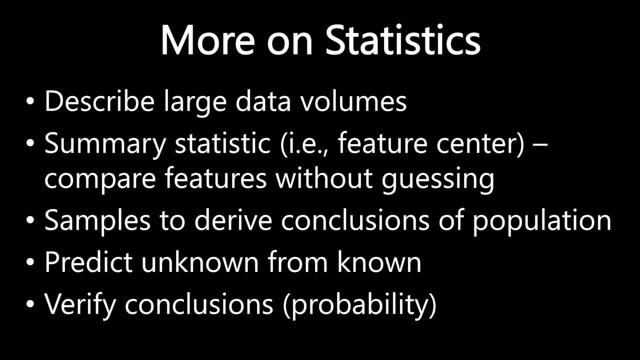 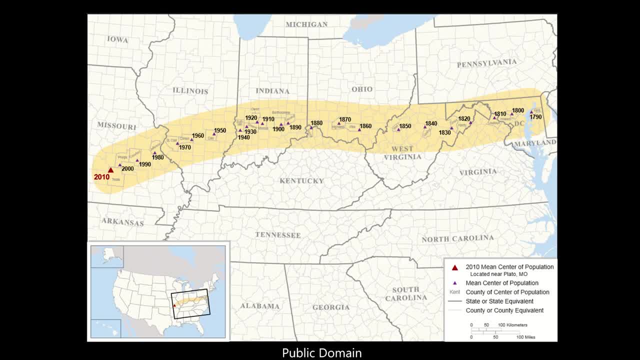 and ultimately finding conclusions through different levels of probability and acceptable risk. For example, this image shows the mean or average center of population in the continental United States and how the mean center has changed since the founding of the country. and how the mean center has changed since the founding of the country. 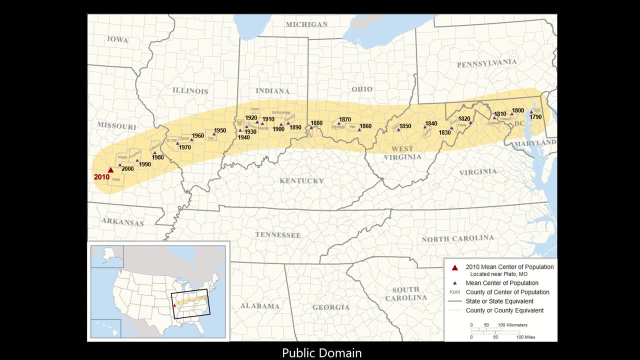 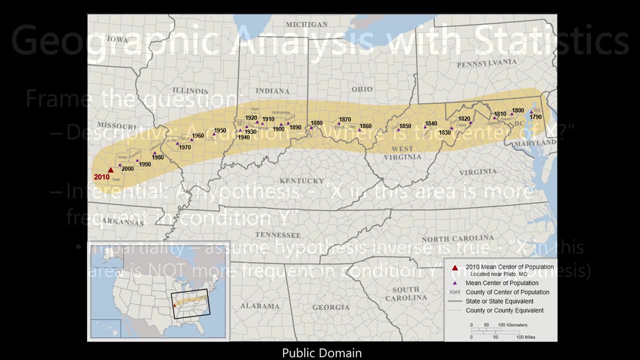 of the country. As you'll note on the far right, the mean center of population in 1799 was centered around Maryland. As populations migrated west in the United States over time, the mean center of population is now in Missouri. Geographical analysis with statistics. 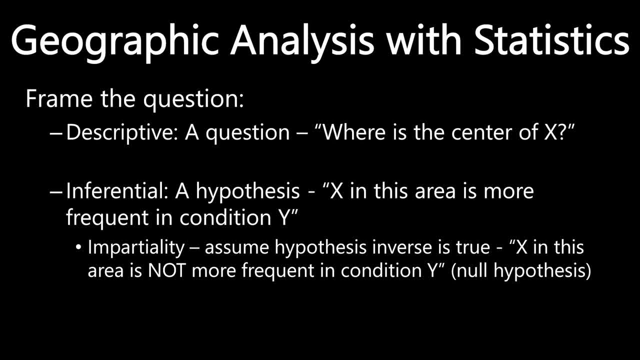 use a similar approach in terms of framing the question being addressed and reaching a conclusion on a basis of evidence and reasoning. For example, a descriptive question such as where is the center of x? Or perhaps an inferential question with a hypothesis you're testing, For example, x in this. 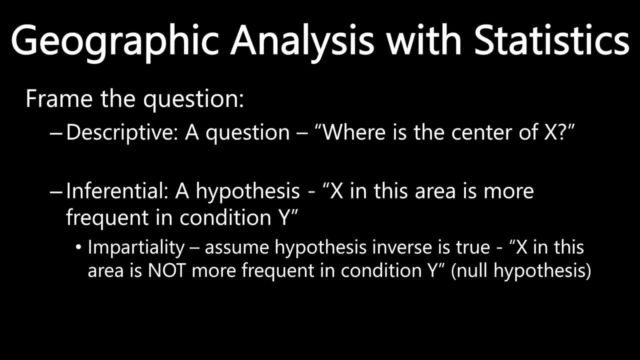 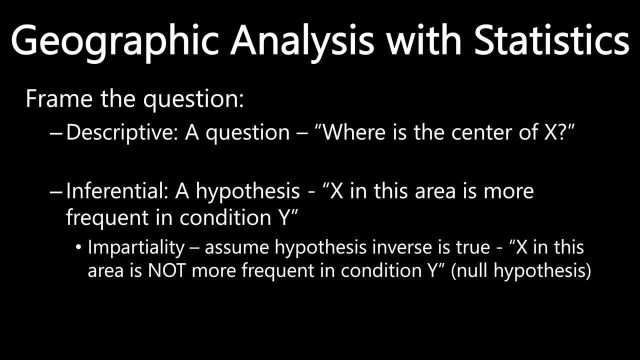 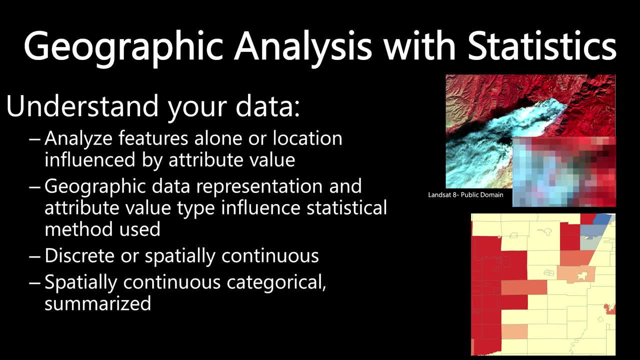 In this area is not more frequent in condition y, or what is known as the null hypothesis. It is important as well to understand the nature of your data. For example, are you trying to analyze the features alone, or how location has been influenced by an attribute value? 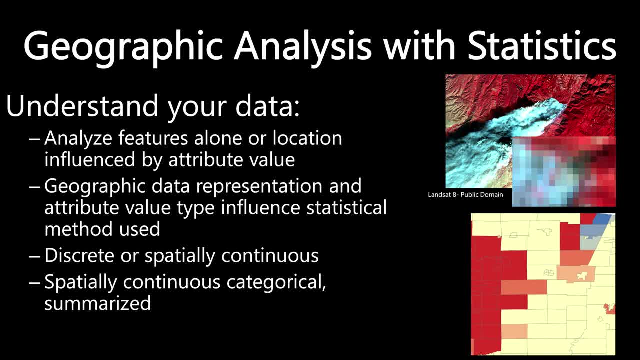 For example, trying to decide where to put a new store, based on the locations of existing stores, versus crime rates in a neighborhood that are influenced by income levels. The type of geographic data representation and attribute value will also influence the type of statistical method used. For example, if your data is discrete, such as point locations or spatially. 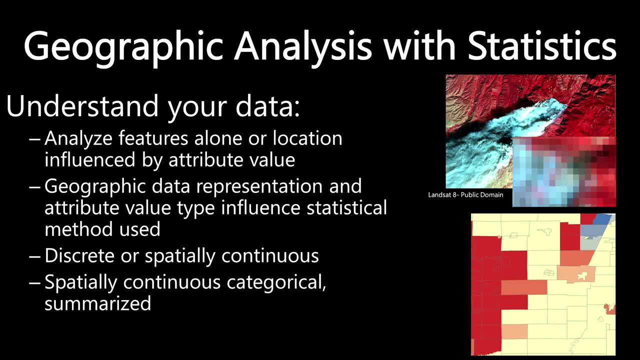 continuous like a raster representation. Additionally, it is important to consider if your data is categorical or summarized. Examples of spatially continuous categorical data could be land cover values. Land cover is continuous and it is assigned to categories as opposed, for example. 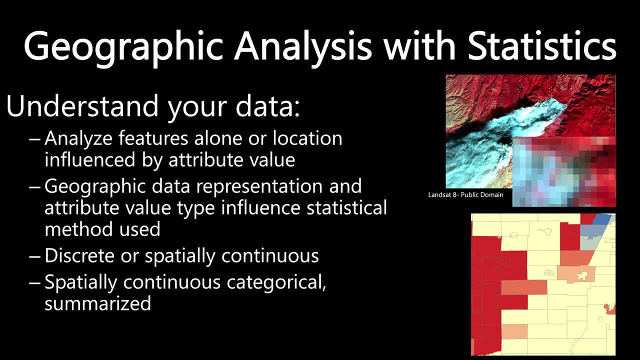 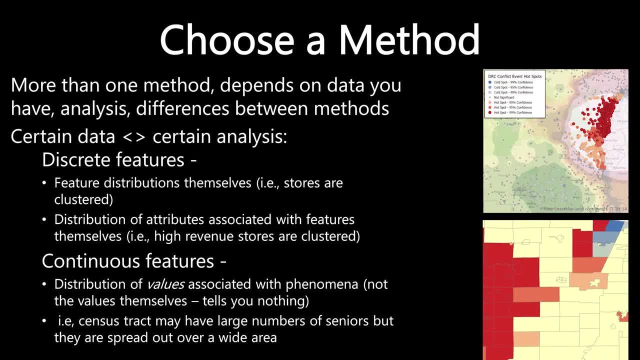 summarize continuous data, like census tracts that aggregate data based on values in arbitrary spatial units. As discussed previously, certain data is not categorical and it is not categorical. For example, if your data is categorical or summarized, such as point locations or spatially. 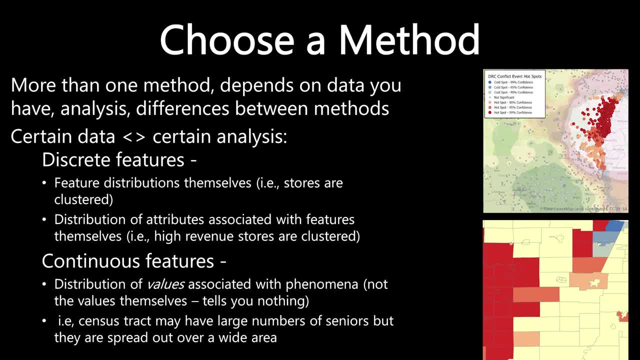 requires certain types of analysis and associated methods. For example, if, looking at discrete features, you are looking at where features themselves are distributed- For example, are stores clustered, Or are you interested in the distribution of attributes associated with the features themselves, For example, 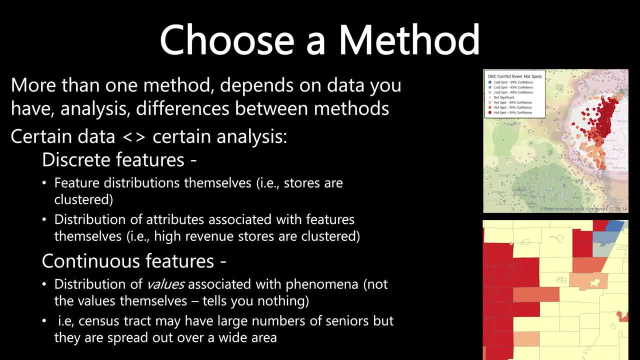 are high revenue stores clustered. This is in contrast to continuous features, where you would be interested in the distribution of values associated with the phenomena, but not the values themselves, which will tell you nothing. As one example, a census tract may have a large number of senior citizens, but 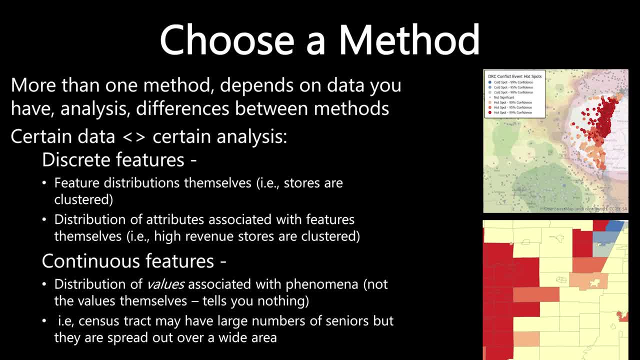 they're spread out over a wide area in the census tract. Just knowing that there's a large number of seniors in one census tract doesn't tell you anything, as you have to look at how the values are related over a distribution in space across other areas. 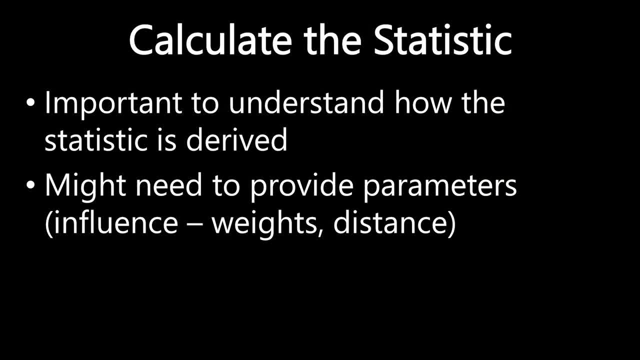 Once you have determined an appropriate method, it is important to then understand how the statistic is derived. Additionally, you may need to provide parameters to the methods being used. For example, are you using weights to determine the importance of a feature or attribute, or what distances are relevant to understanding the statistic? 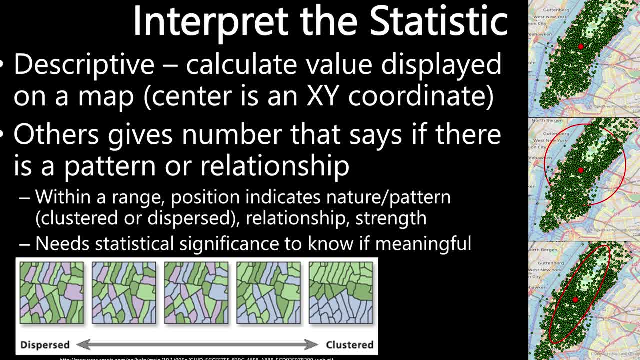 An important component of using spatial or other statistics is how you interpret the statistics. that was derived from the method chosen. In the case of spatial statistics, you can use an interpretation based on description, For example, using a map to show the center coordinate of a given. 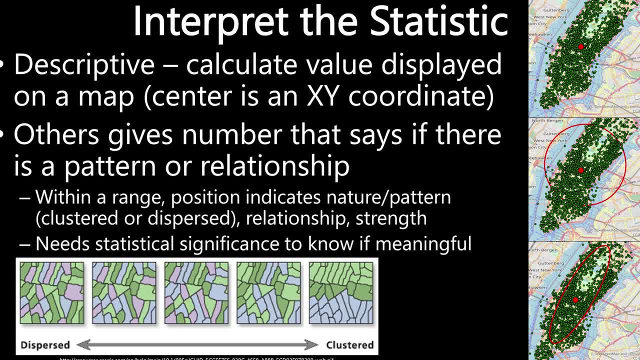 phenomena, like the median population center shown earlier in this lecture. Like other statistics, spatial statistic methods will give you a number to determine if there's a pattern or relationship. For example, are your phenomena clustered or dispersed and what is the strength of that relationship? Finally, you'll need to know the level of 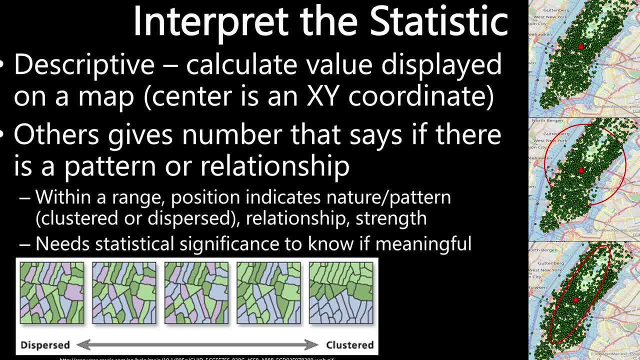 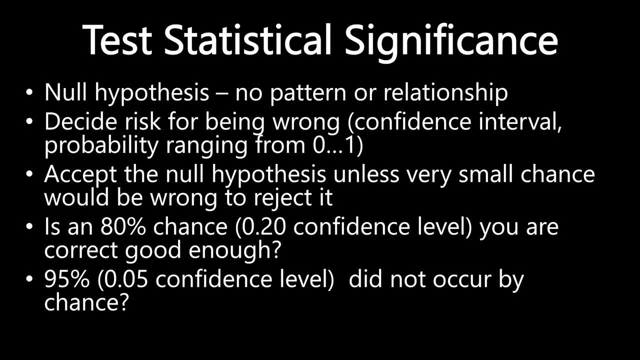 significance in order to determine if the output of your analysis is in fact meaningful. Spatial statistics also do tests of statistical significance. For example, do you accept or reject the null hypothesis that your analysis is correct? For example, do you accept or reject the null hypothesis that your analysis is correct? For example, do you accept or reject? the null hypothesis that your analysis is not correct? For example, do you accept or reject the null hypothesis that no pattern or relationship exists? If you're a heirloom, you're the heirloom of historical statistics analysis methodology. All your items or variables matter and you best prefer to restrict your hypothesis and 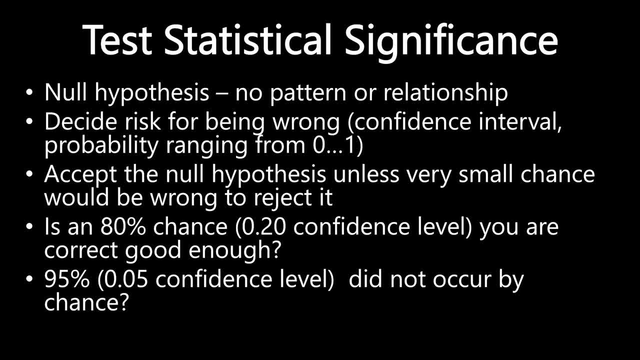 gesture. Ultimately, you're deciding the level of risk for being wrong with your hypothesis. This is what is known as a confidence interval, which is a probability value ranging from zero to one. For example, is there an 80% chance you are correct and is this good enough? 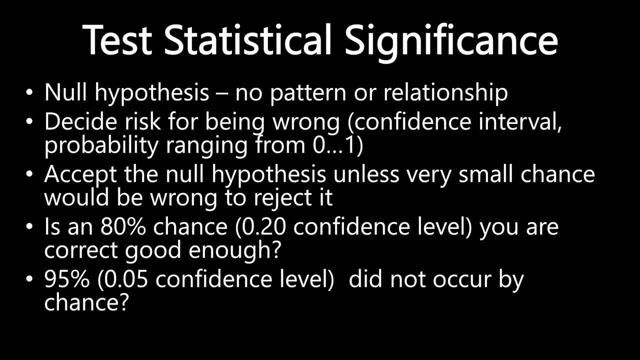 given for what you are analyzing. A very common confidence level is the 95% confidence level within a given hypothesis. This is when a no-compищente hypothesis is collected and adjusted against the same criteria. Incre occurring confidence as gegeben by not-ive models, be it probability levels, placement, jard, lime, chestlet, overlay, etc. 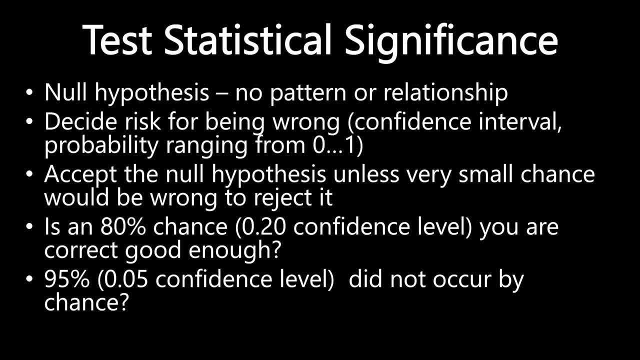 level that things did not occur by chance. Spatial statistics software run appropriate tests for the initial statistic for you to compare with a critical value based on the confidence level to determine if the results are statistically significant. If the test statistic exceeds the critical value, you can then reject the null hypothesis and state that the results are statistically. 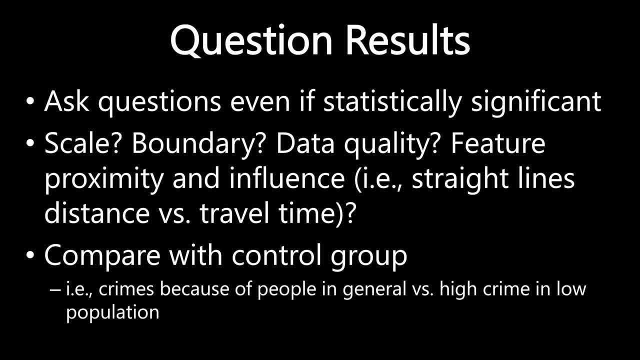 significant. Some examples of things you should do to question your results, even if your data comes back as being statistically significant, include examining the scale of your analysis, boundary and edge effects, data quality, proximity and influence, such as straight line distance versus travel time. 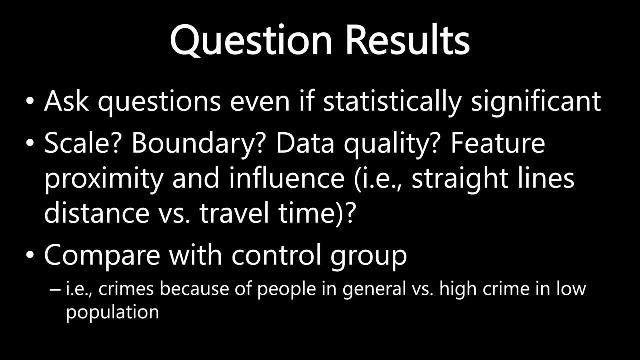 distance. Furthermore, you may need to make comparisons between the results of your analysis and the results of your analysis One jeden한다 battering point in time. management depends on your chickens report and their結果. In this given scenario, you can make comparisons in: 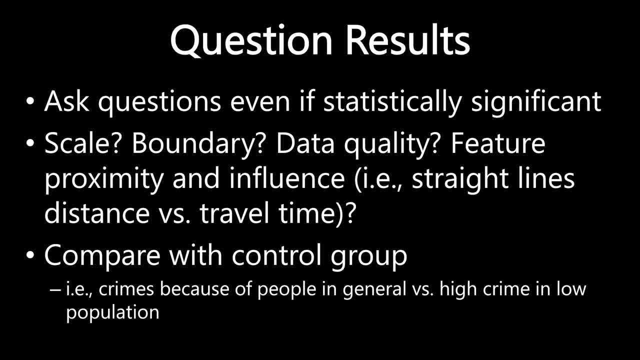 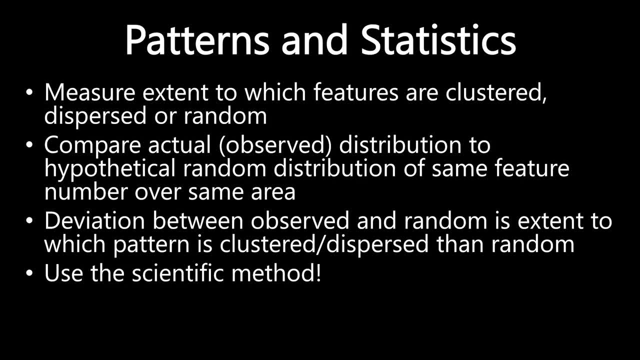 open distance models that there are nothese, that show the poor collection of picture in the detail of a raczym data set or find a Human Dosage. Another important aspect of spatial statistics is understanding the patterns that are created. For example, are your features clustered, dispersed or random? 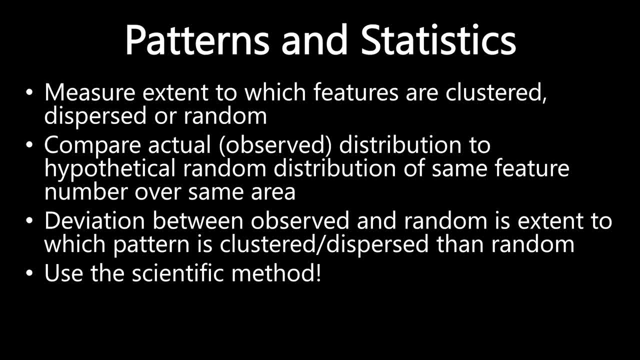 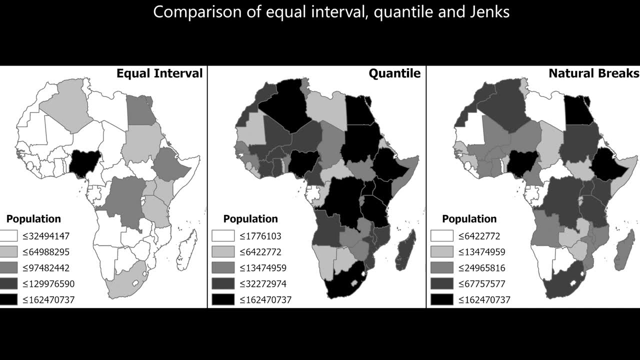 patterns have to be compared with a random distribution of features over the same area to determine if the phenomena are statistically significant or simply by chance. For example, looking at map observations alone is not good enough. Thematic maps can easily be manipulated based on the statistical classification method used, like seen in these maps that show the 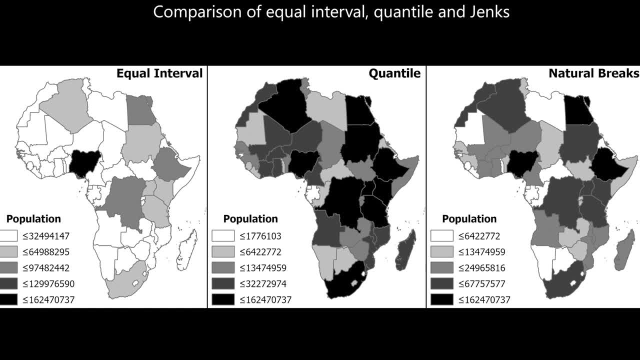 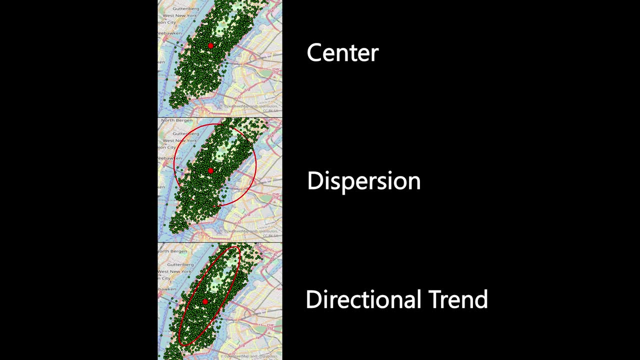 population of Africa using different display strategies. It's all the same underlying data, but looks different simply because each map is using a different display strategy. These images show how you can evaluate the results of spatial statistics. Specifically, these images show examples of the center feature as seen in the top graphic. 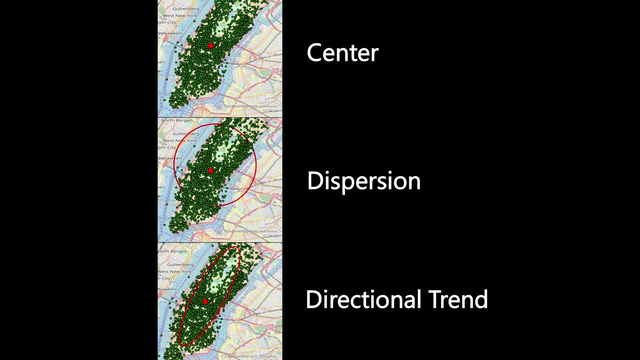 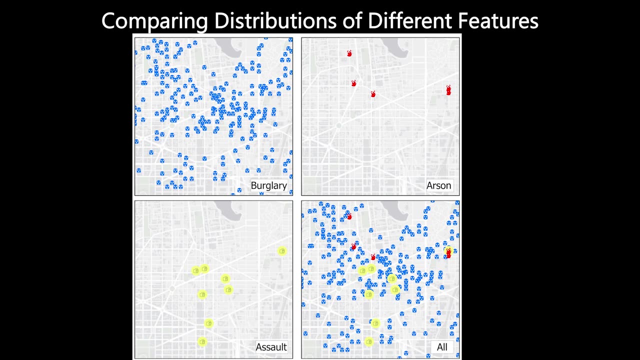 the dispersion of features around the center, or compactions, as seen in the middle of the graphic, and directional trend, as seen in the bottom graphic, with an ellipse showing the overall directional trend. And finally, distributions can be used to compare different feature sets. For example, this image shows comparing burglary, arson and assaults to compare distributions of these types of crimes in a given study area. 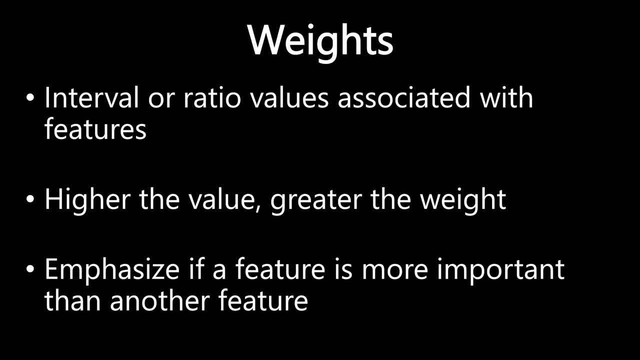 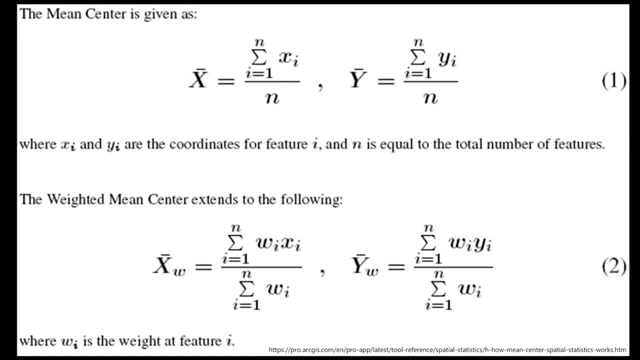 Finally, another important aspect of spatial statistics to mention in this introductory lecture are weights. Weights can be used to emphasize if a feature is more important than another feature. Here are the formulas used for the mean center and weighted mean center. The basic idea is that the x and y values of a feature coordinate pair are averaged. 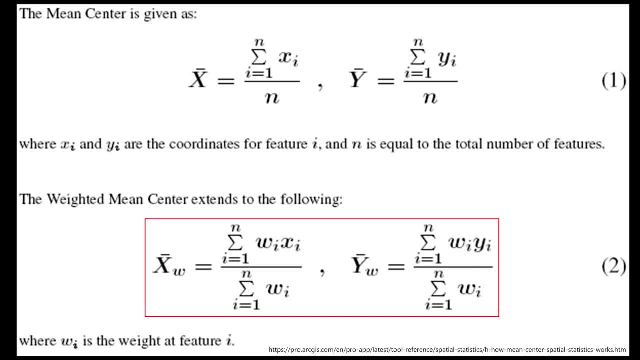 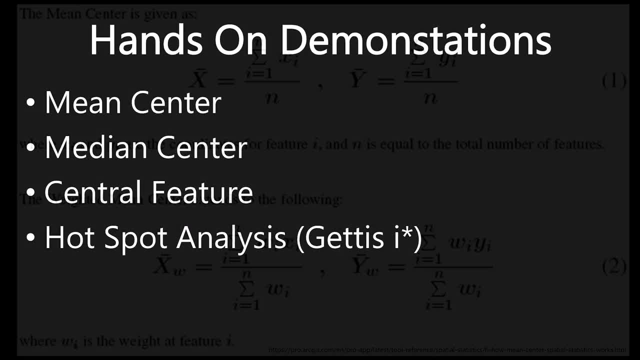 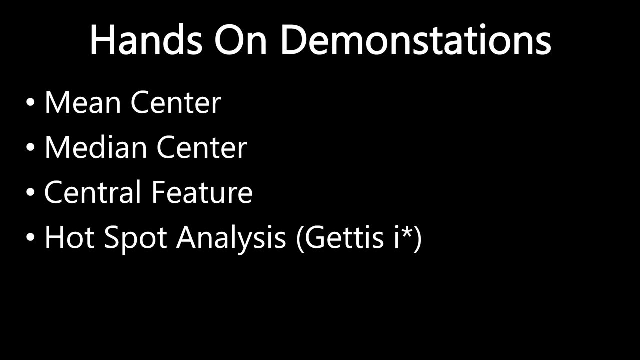 However, a given feature is not a function of a feature coordinate pair. A given feature can be given more importance or weight, just like is done in a weighted non-spatial average. I'll give you a hands-on demonstration of some basic spatial statistical methods as available in the ArcGIS Pro software. 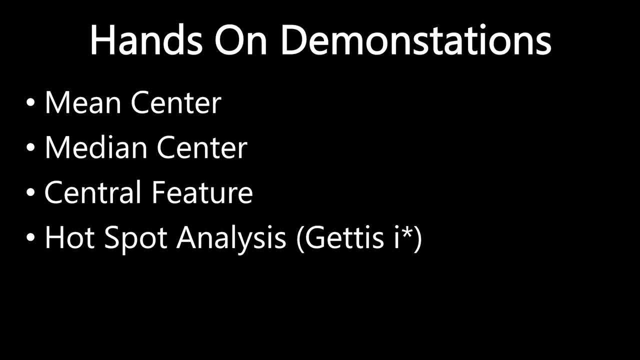 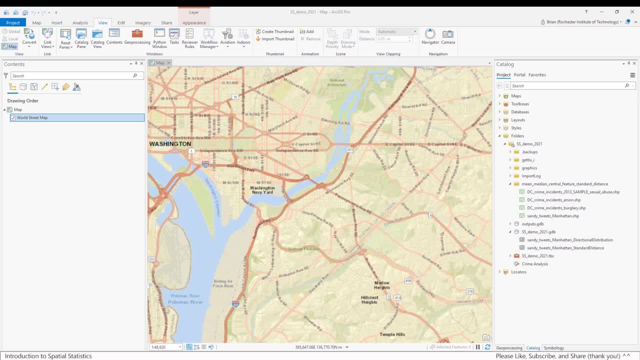 Datasets used in this demonstration are available in the video description below. Welcome to the hands-on demonstration part of this introductory lecture to spatial statistics. I want to briefly show you some of the basic methods available to you in the ArcGIS Pro software as a follow-up to some of the concepts that you learned about earlier in this video. 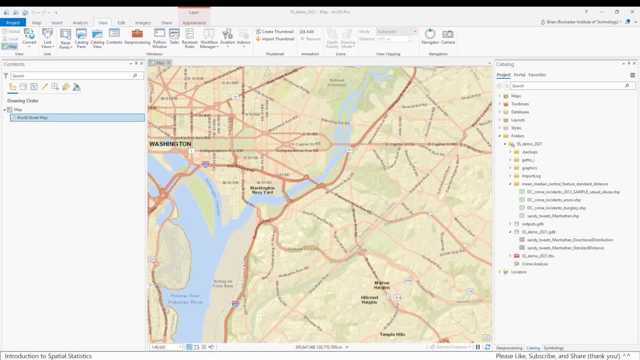 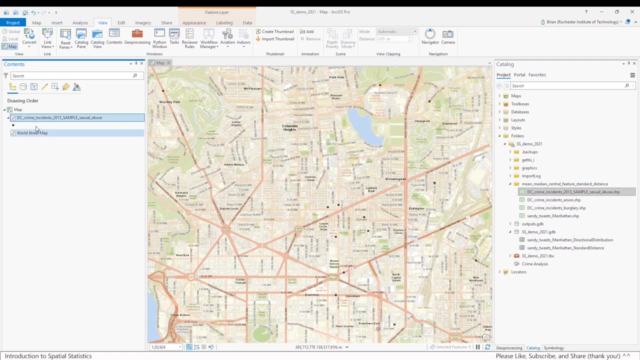 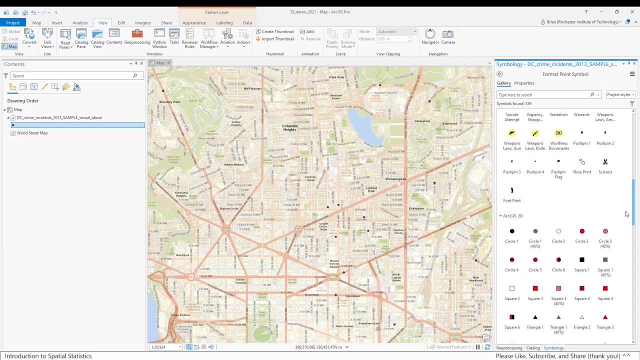 Let's start with mean center and to demonstrate that I have some data related to assaults in Washington DC in the United States, So I'm going to pull a shapefile of assaults in and I'll change the color to make it more visual and and. 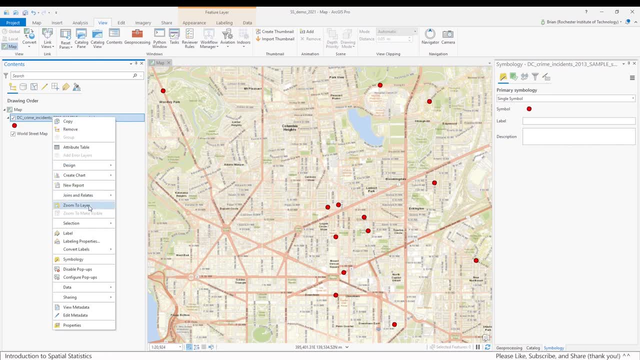 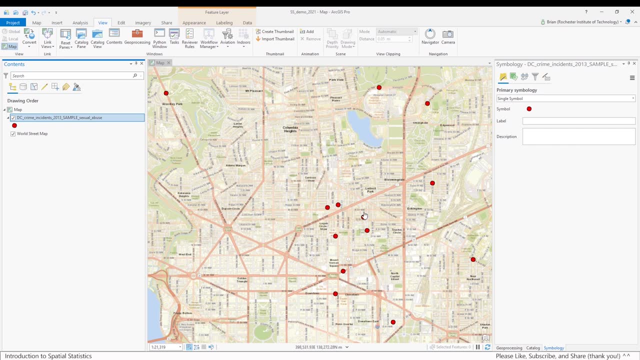 I'll zoom to the extent or zoom to layer. So right now you're seeing the extent of all of these assault cases from this dataset, and so what the mean center is going to do is determine the average, based on the XY coordinate values, of these points. 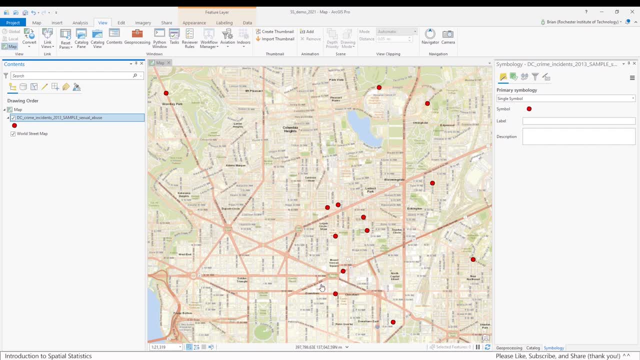 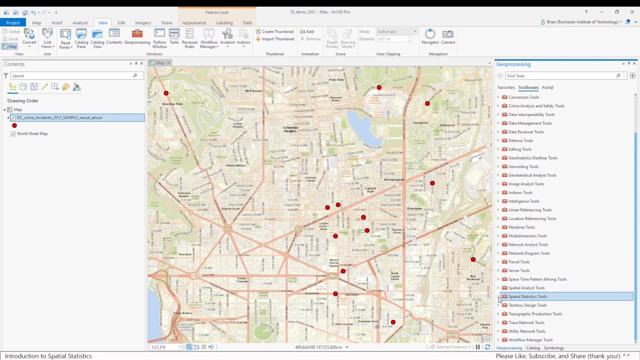 to determine where is the center and where is the stay center of this data set And to use spatial statistics tools in ArcGIS Pro. a good way to learn how to access them is go to Geoprocessing Toolboxes- Spatial Statistics Tools- and I'm going to be using a lot of the Measuring Geographic. 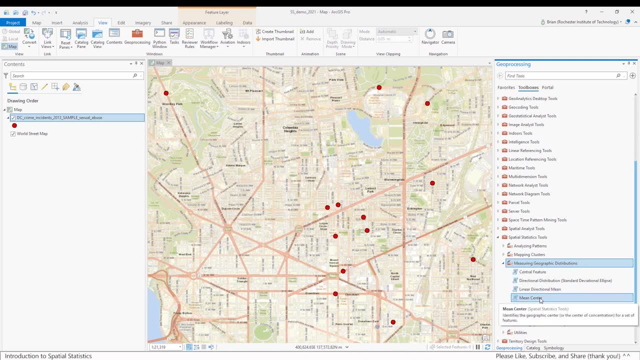 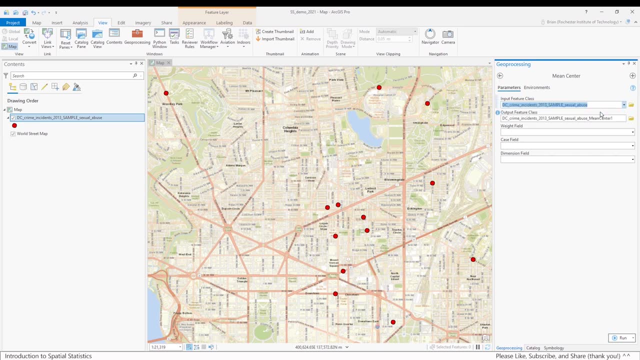 Distributions And here we have Mean Center and it's pretty easy to use. I select the Assault Cases. I'll just take the default Now. earlier in the lecture I talked about a weight field. This is where you could have values from the 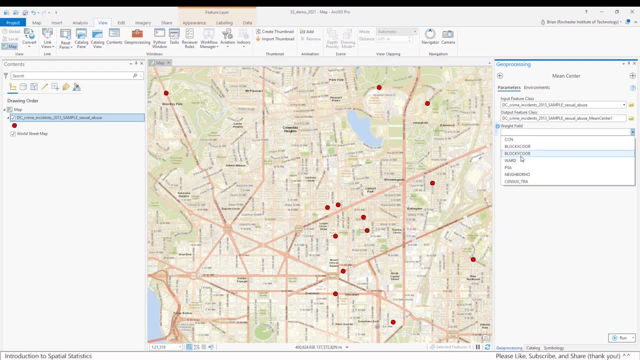 feature classes attribute table be used as a weight when calculating the average. I'm not going to do that, but I just wanted to make you aware of that as I did talk about that previously. I'll ignore the other two and I'm going to 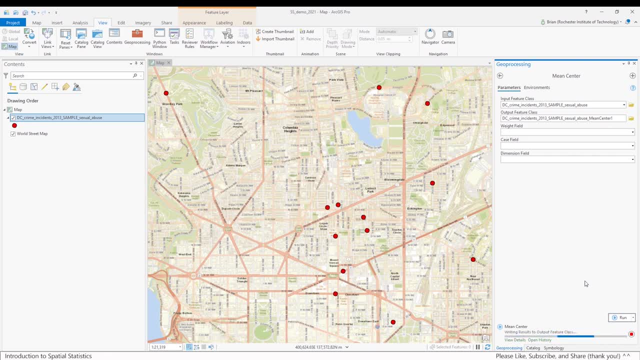 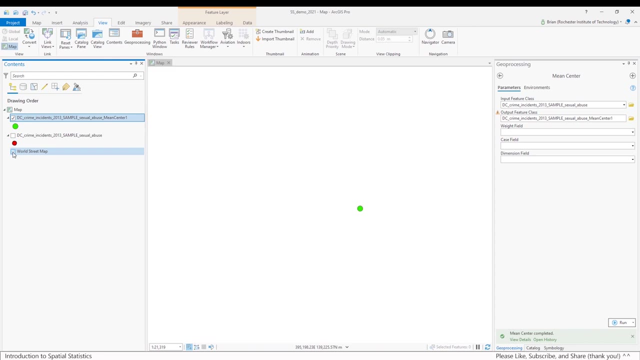 run this And you can see this green point that showed up, And so what this green point is is the spatial average of all of these other points. So, again, a good introductory way to get started if you're brand new to spatial statistics. 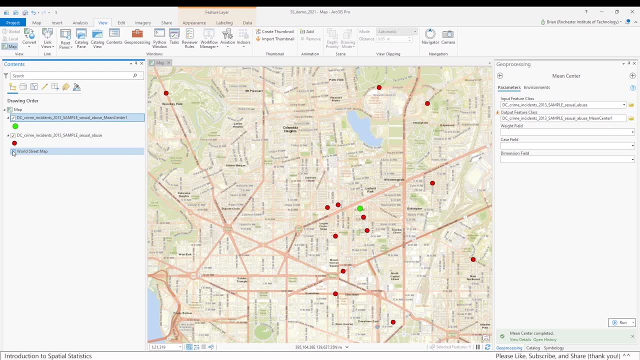 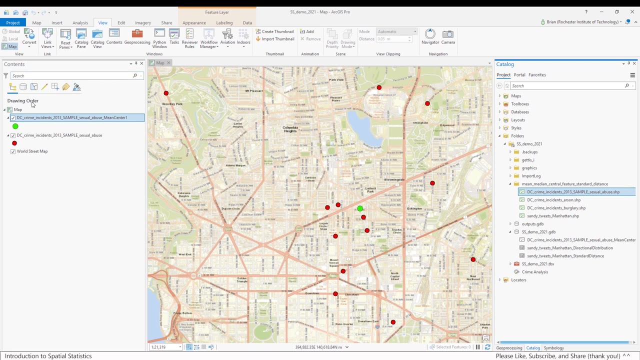 Let me next show you now the Median Center. You would use Median Center when you need a tool that'll measure the central tendency of data that is robust to spatial outliers. So, for example, if I'm doing crime analysis, I might have a hypothesis that arson, which I'll bring. 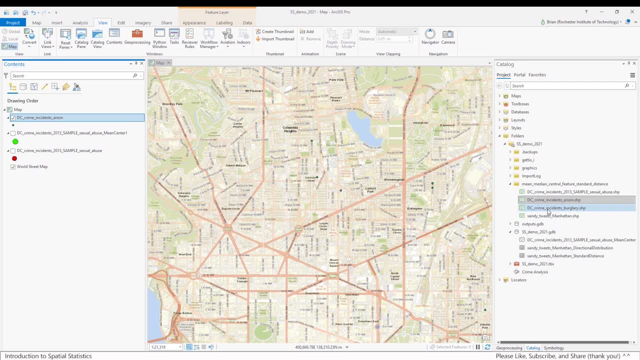 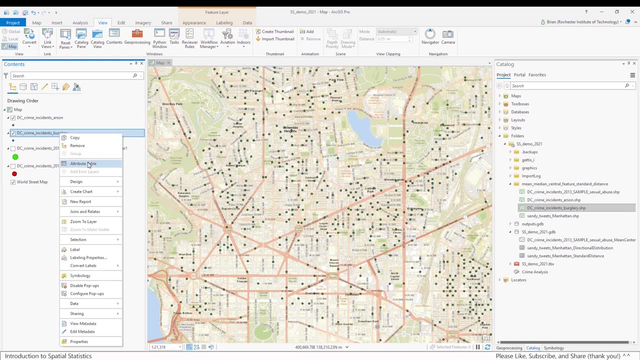 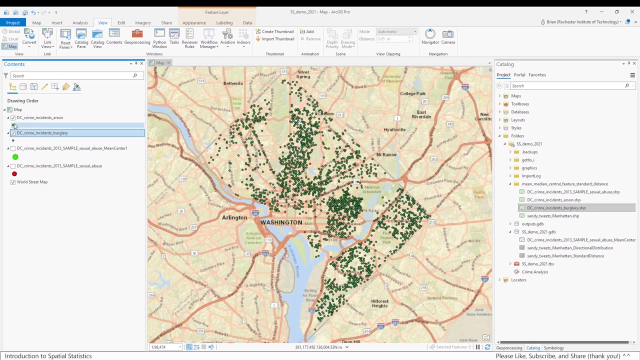 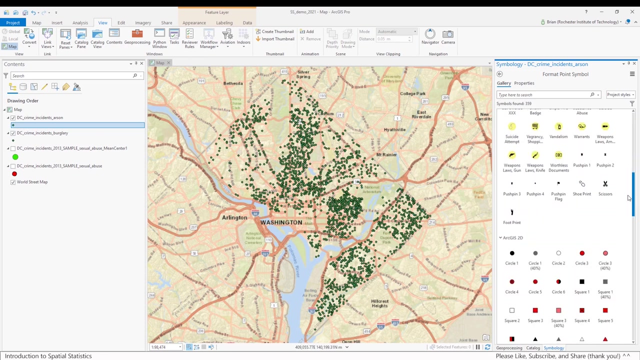 in now and burglaries perhaps have some type of relationship. You can see there are many, many more burglary points compared to arson points, and let me just change this to make it a little more visual. So I'll make the arson points a red circle. 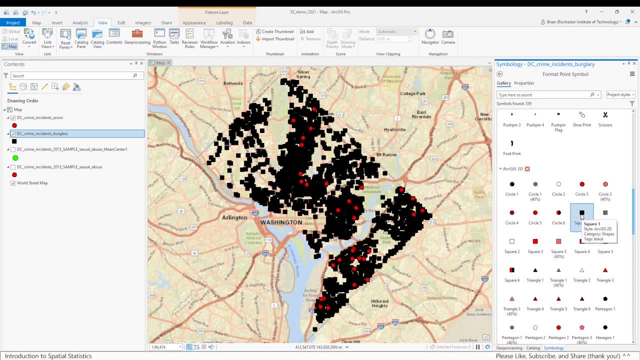 and I'll make the burglary points green and you can see here that the red circle points- black squares map gets a little cluttered when you do that, but you can see there's a lot of burglary points off to the northwest here and so forth, so I 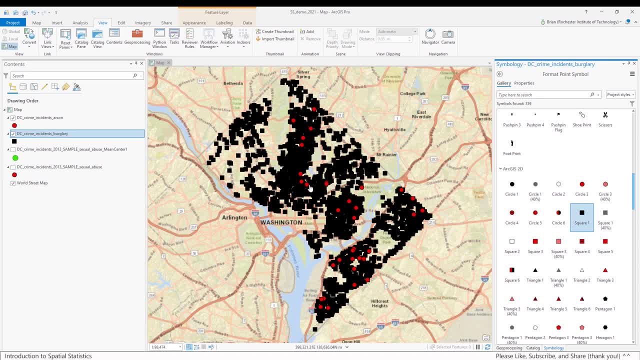 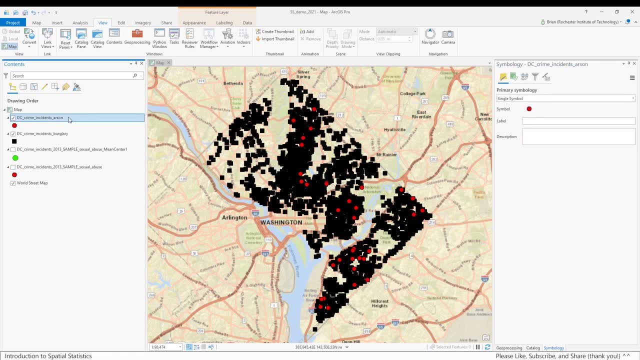 really want to make sure that peripheral events are not affecting this analysis, I'll do so. I'll first run median Center on the arson points and it's a very similar type of tool, like the mean Center that you just saw. I'm gonna go back to geo processing and it's right here, right underneath mean Center, and 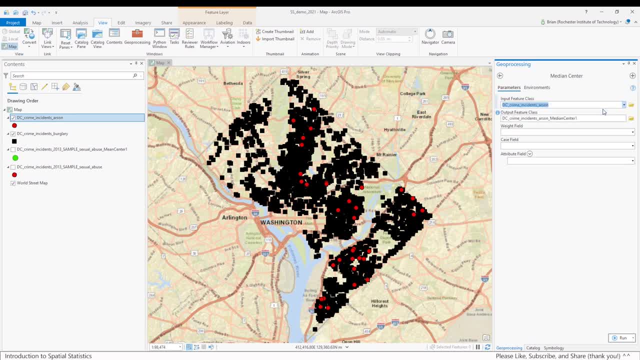 very similar workflow, so I'll select arson. I'll take the default. you have a weight field, like we talked about earlier. I won't bother with the other two for what I'm trying to do here and I'll run it model. I'll just rotate the original one to get the real picture. so let me just 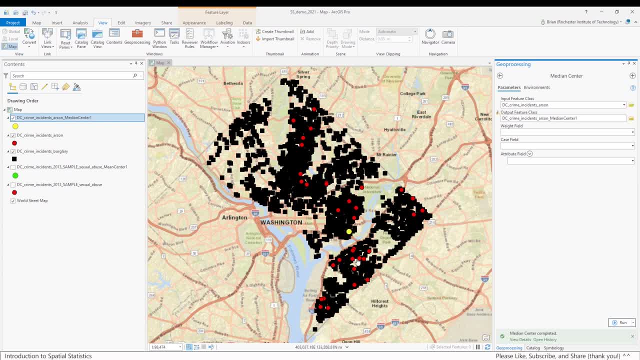 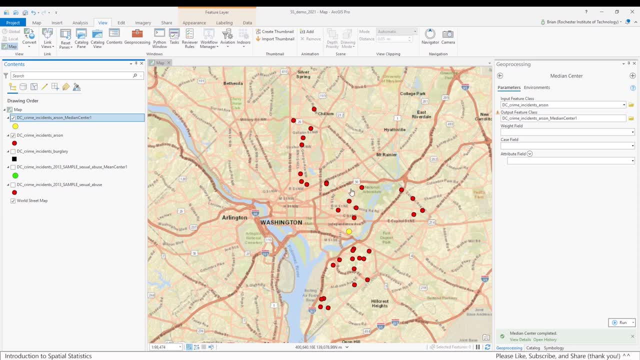 make sure that you forget to do that actually. okay, you can see gray arson points are below, as the way that thisButton is 抓бшая to, gsmkU tv pretends to, and so we see this yellow point now. so this is the median center of the arson. 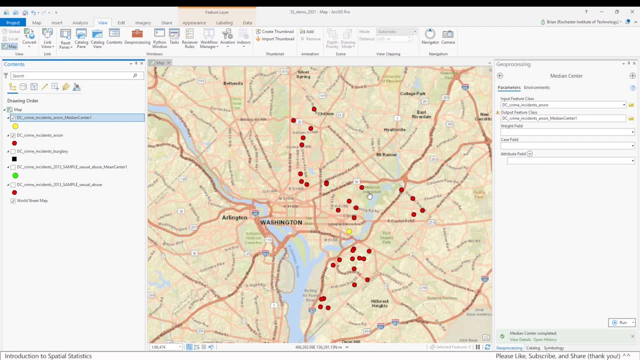 data. so the arson points are these red points and their median center. again, this isn't an actual spot where an arson happened, it's simply just spatially the median center of the distribution of these points. okay, now let's run the tool on burglaries to look at the来. 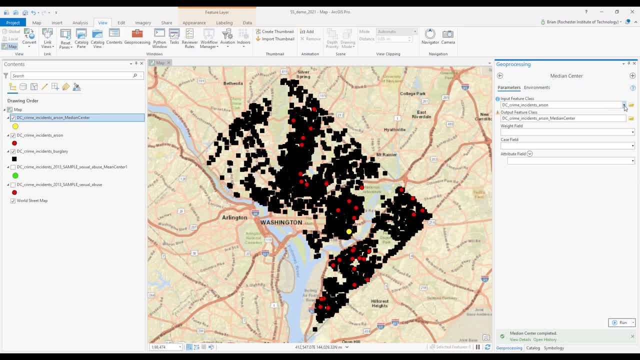 filho, their median center. I already have the tool open, so I'll select burglaries from the drop-down. Now just make sure that you rename the file. I actually made a little error when I was preparing this. I'll get a different feature: class name Again. you can select a weight, and so. 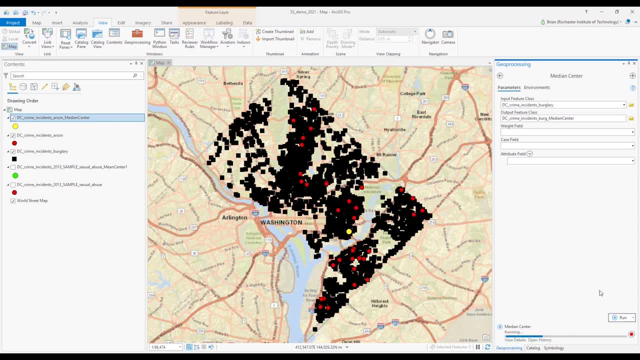 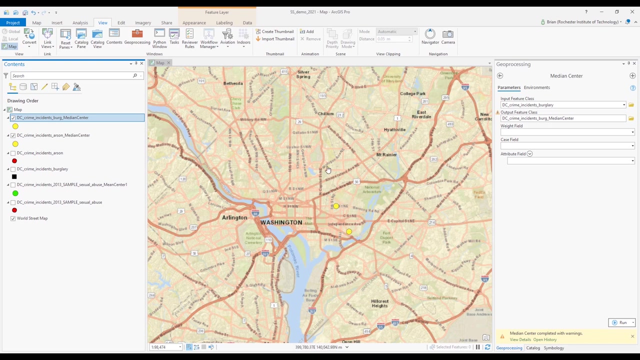 forth, I'll hit run. So now, the two yellow dots represent one. the first one is the burglary median center and the other one is the arson median center, And this can give you a sense of how these features are distributed over space. Now, remember, as I 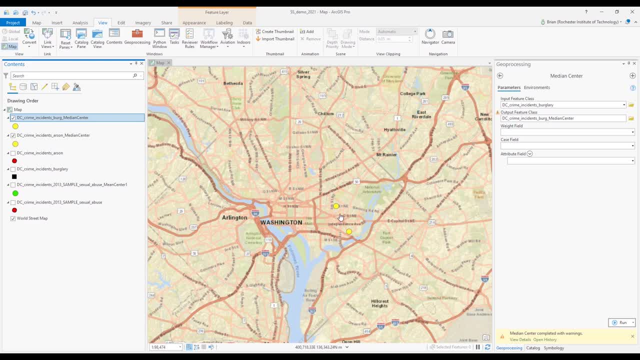 said previously, these aren't the actual locations of specific arsons or burglaries. These are the locations of specific arsons or burglaries that are just their sort of spatial median within the overall study area. So let me show you now a basic method that can determine a specific feature and that 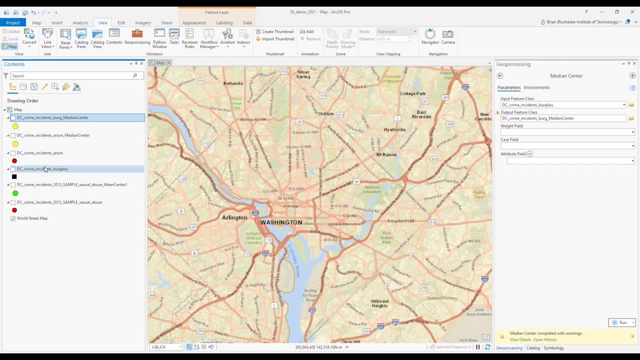 will be central feature, And the central feature uses an approach where the total distance from every feature to every other feature is determined and the feature with the lowest total distance is determined. And to do that we'll go to a completely different study area. 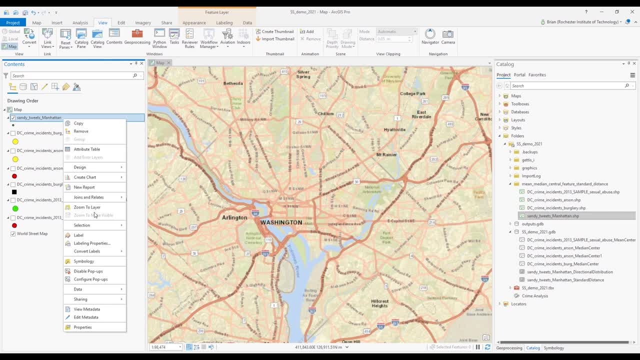 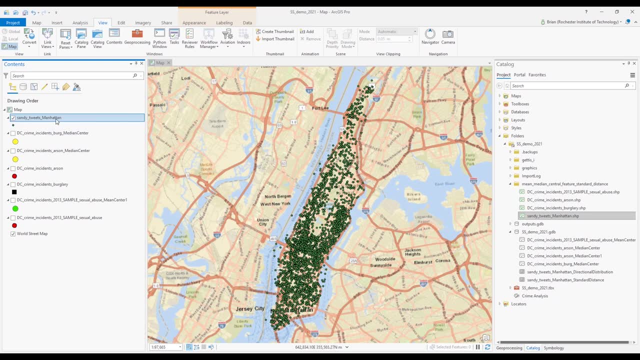 We're now going to go to Manhattan in the United States And these are tweets from Hurricane Sandy that happened in 2012.. And it's a good representation of what's going on in the United States. And it's a good representation of what's. 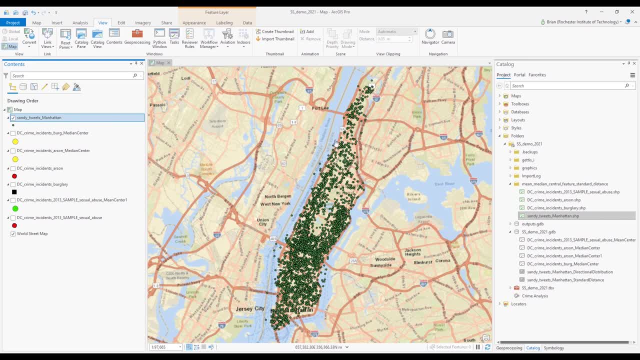 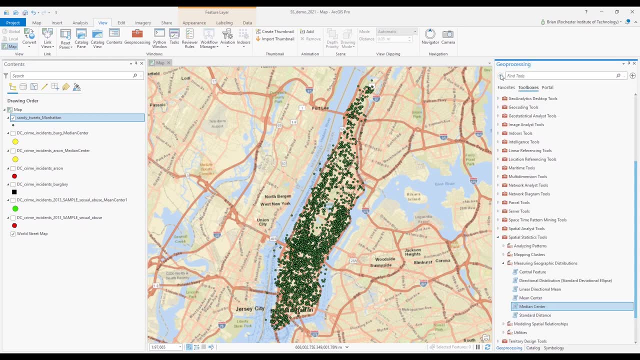 going on in the United States. So these are the search results And these are the data points that I'm going to be showing you now, And then I'll use the actual data reports to determine where the central feature within this overall data set may be, And so to determine that I'll go back to toolboxes spatial. 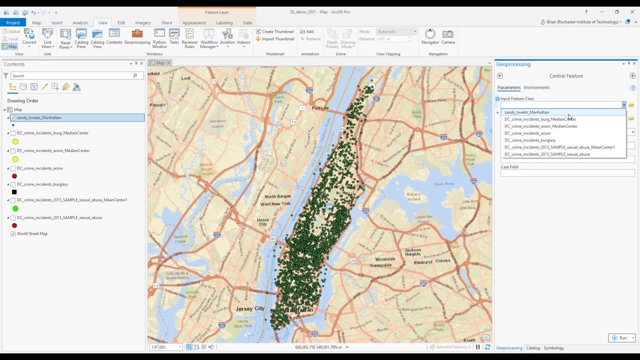 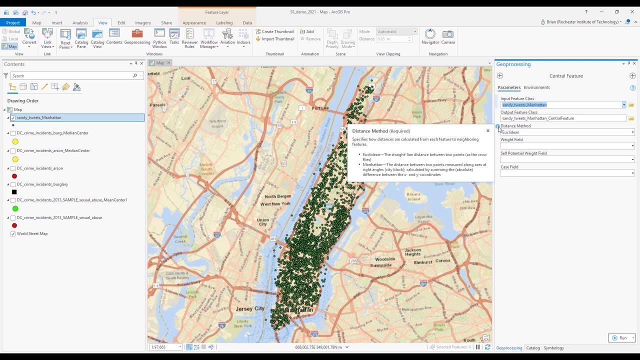 statistics measuring geographic distributions, and I'll select central feature And in this case, the input will be the Sandy tweets. Take the default. Now Determining how distances between things are are calculated and this can have an effect on The final output, and this was something I mentioned earlier in the lecture part of this video. I'll take the default Euclidean. 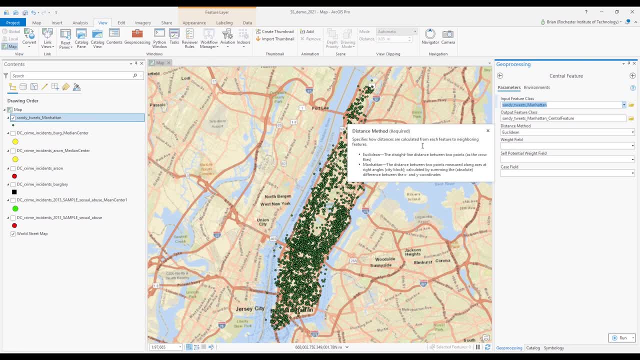 I don't have time to really explain all this in this video, but this is something to follow up on if you plan to really do more with spatial statistics. and Again, I have a weight field and some other Parameters that I can set that I'll ignore. 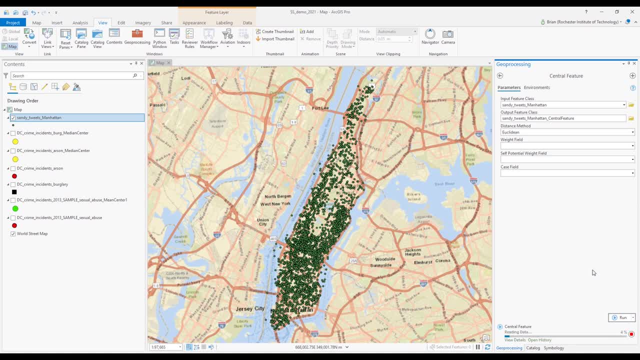 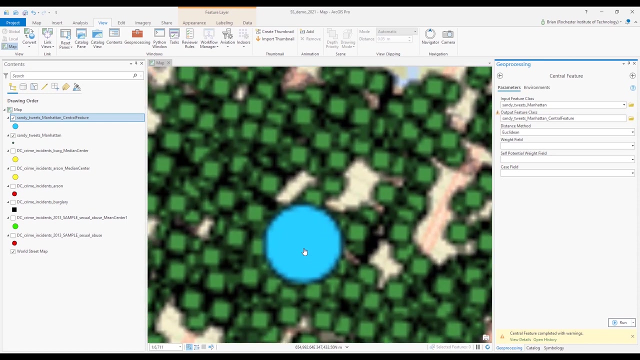 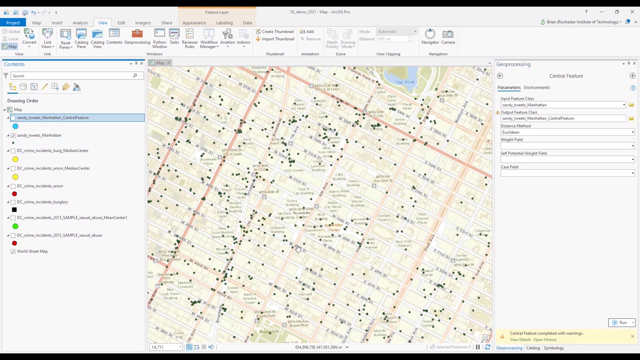 Because we're doing a quick demonstration here Now. this tool. you can see this blue dot. this represents the central feature. This is, in fact, where one of the tweets are. I Didn't turn it off, But if you zoom in a little closer you can see this green dot here. 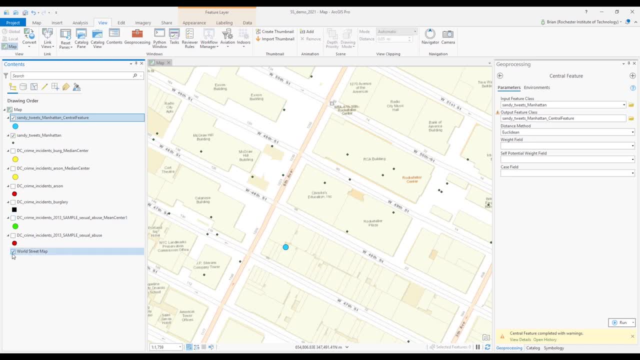 That is the central tweet compared to all of the other tweets that are in this data set. Okay, let me finally give you a quick introduction to hotspot analysis. this is actually a pretty big topic and I encourage you to learn more about it. beyond this quick demonstration, I'll do: 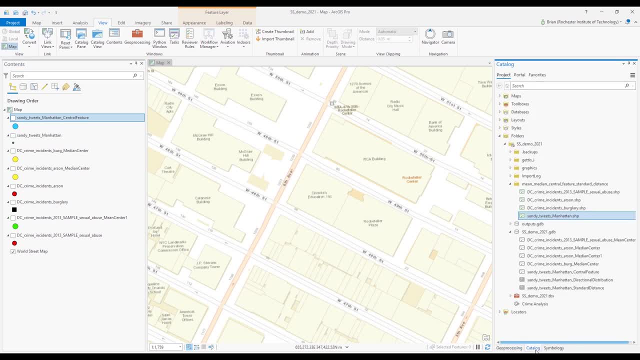 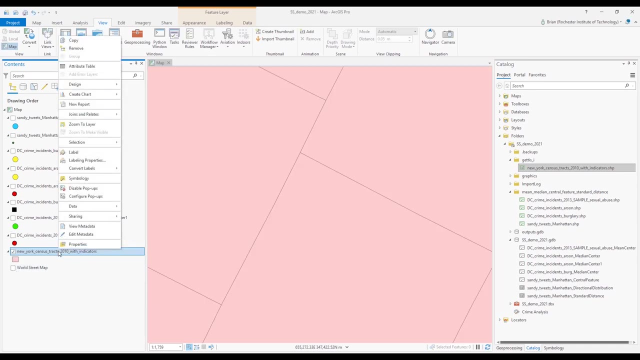 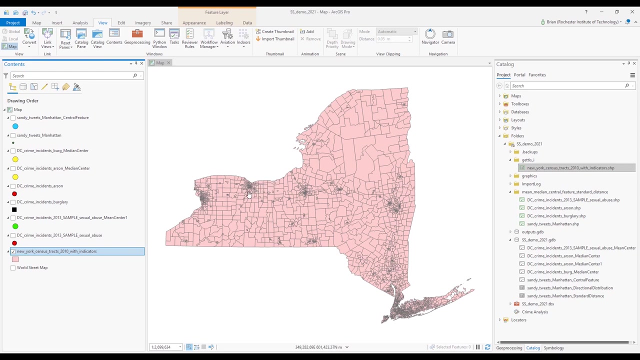 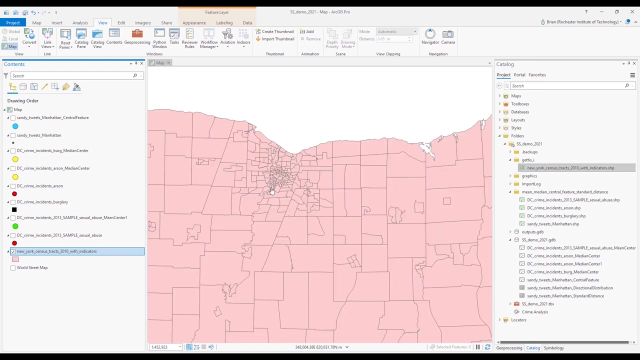 To set this up. I'm going to bring one more new data set in Here. you're now going to see census tracts from New York State here in the United States, where I live, And what I'm interested to know is: are there clusters based on attribute values and this: 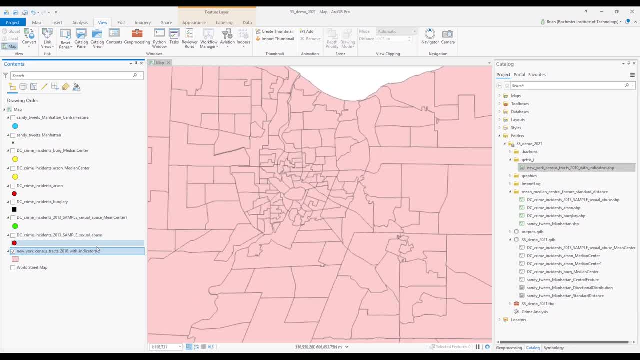 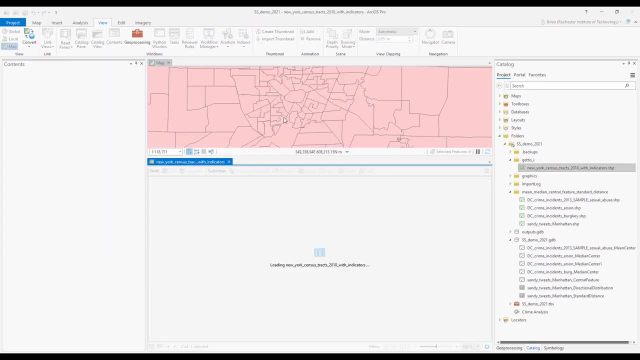 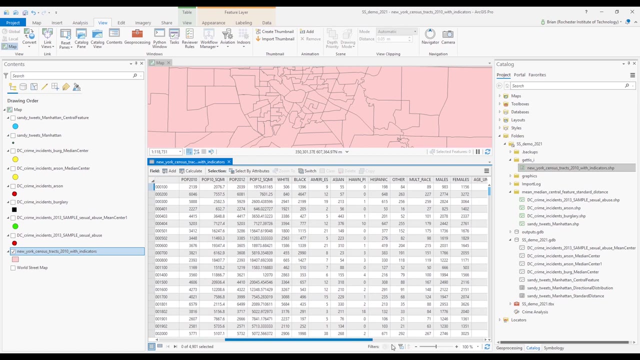 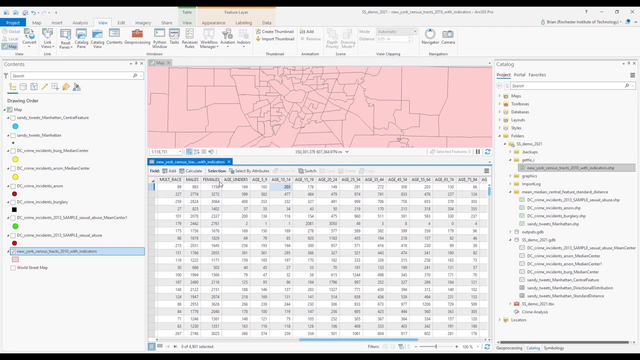 ties in directly to many of the topics I talked about earlier. If you were to look at the attribute table, you can see I have a lot of census indicators inside of this data set And census bureaus, not just the United States, collect this kind of thing. The 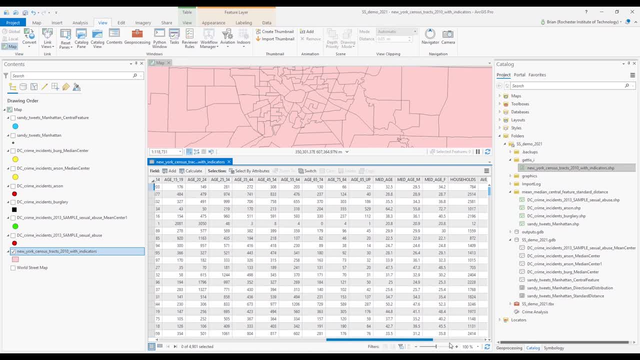 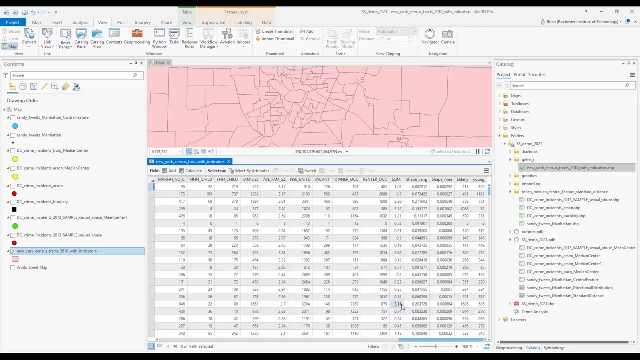 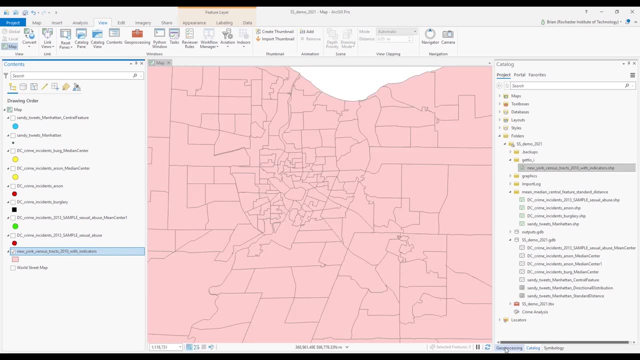 age of people who live in a census unit, ethnicity and so forth. So in my case I'm curious to see, looking at all of New York State, if there's any particular types of clusters of elderly people And to run this tool. I'm going to go back to 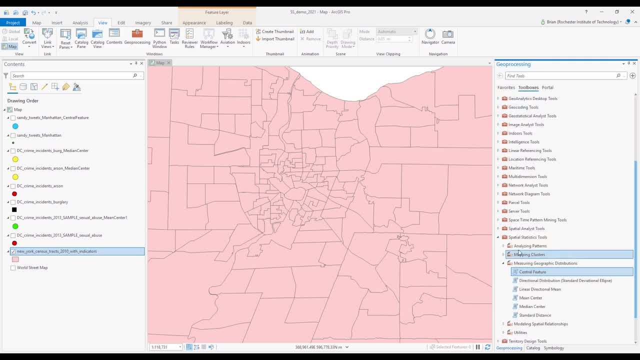 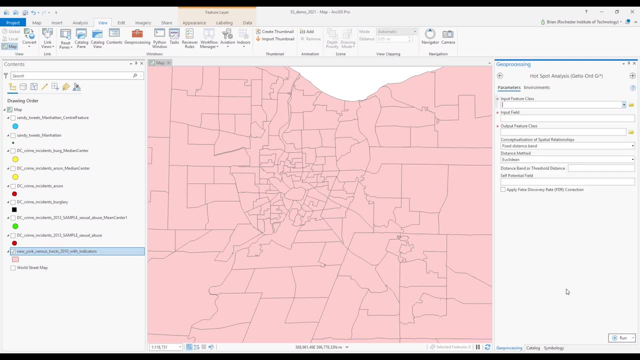 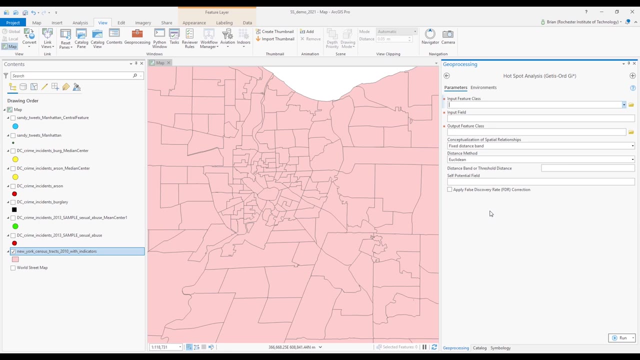 Geoprocessing, and this time I'm going to go to Mapping Clusters, Toolset, Hotspot Analysis. Now, something I should mention is Hotspot Analysis is not the same as a heat map. A heat map looks at the frequency of features in a given area. 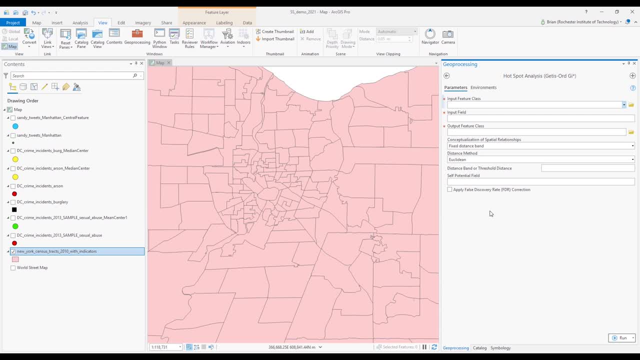 where Hotspot Analysis is looking for statistical significance of clusters. Now, like I said, I'm doing this really quickly just to give you an introduction. I do have other videos on my channel where I go more in-depth on Hotspot Analysis and more of the technicalities. 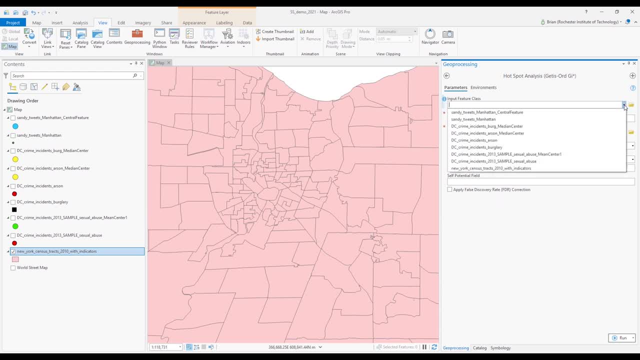 behind it, but I'm going to go ahead and do that now. So I'm going to go ahead and select my census tracts. I'll select elderly. I'm interested in clusters of elderly. I won't have time to discuss any of this really, but here's another. 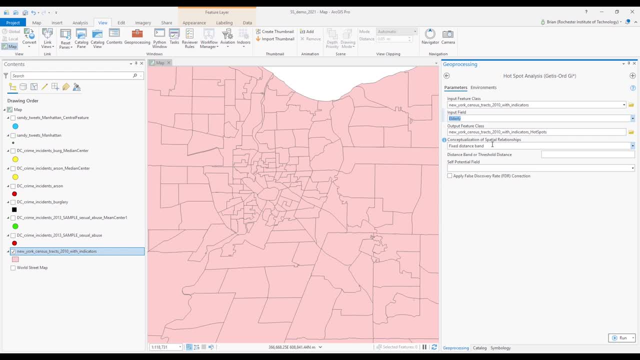 example of when you're determining a method to do statistics, you have to think of how the statistics are going to be used. So I'm going to go ahead and select how the statistics are going to be used. So I'm going to go ahead and 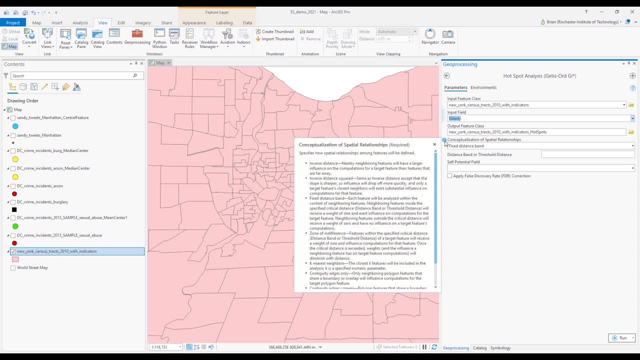 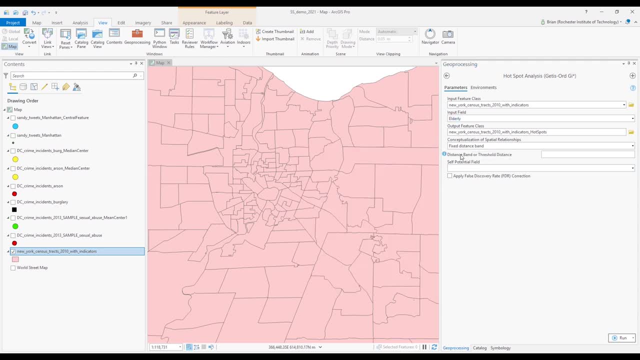 the relationships, or the conceptualization of spatial relationships are done- inverse distance and so forth- And there's actually ways that you can compute this, even determining the distance band and threshold radius, sorry, the distance band and threshold distance. There's ways that you can calculate that. 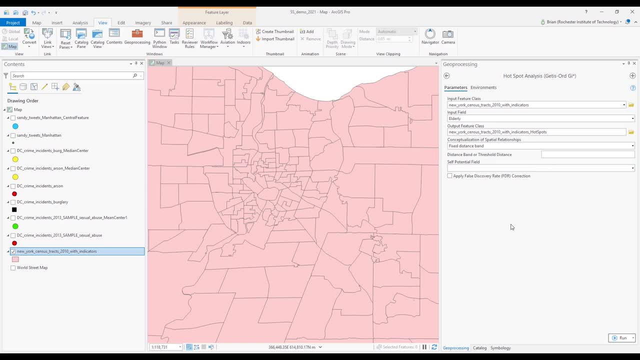 but you can also use the tool frankly, at a superficial level, like I'm doing, where the software will calculate those things for you automatically. And again, I just want to show you how this tool looks like in practice. So I'll hit run, and ArcGIS Pro has gotten really good with sort of helping you. 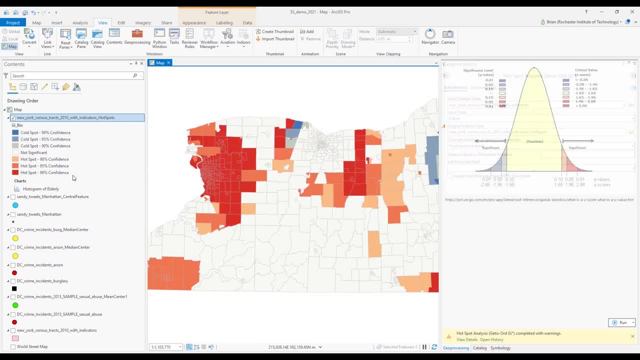 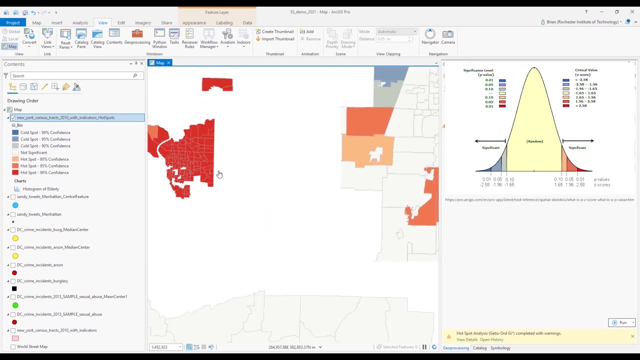 So you get the results come out, and here you can see the software automatically generated a visual representation telling you hotspots in the different confidence intervals, not significant, and then cold spots, And so what this is telling you is that there are clusters of elderly people. 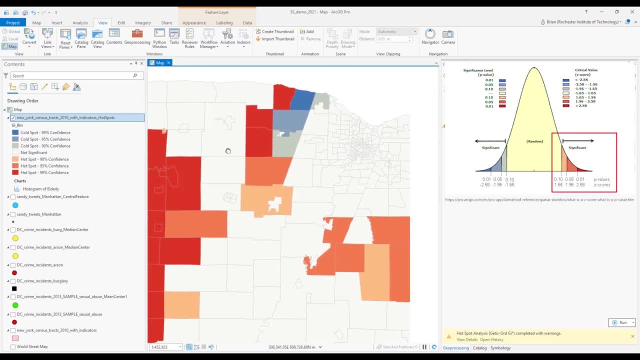 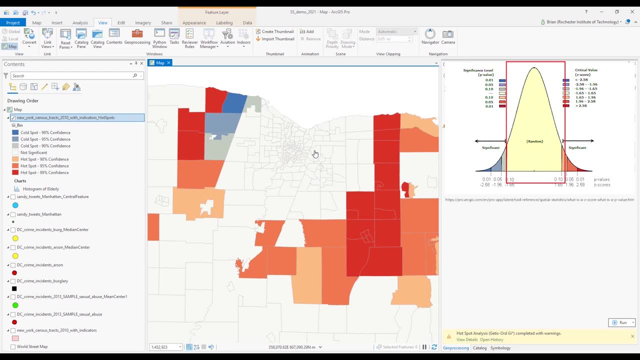 This is a city called Buffalo, a lot in the urban. Now this is where I live, around Rochester, New York. It's interesting that there are not a lot of elderly people living inside the urban core, but these are the suburbs where there are. 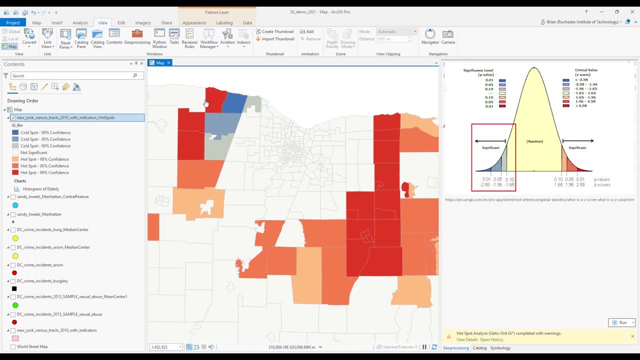 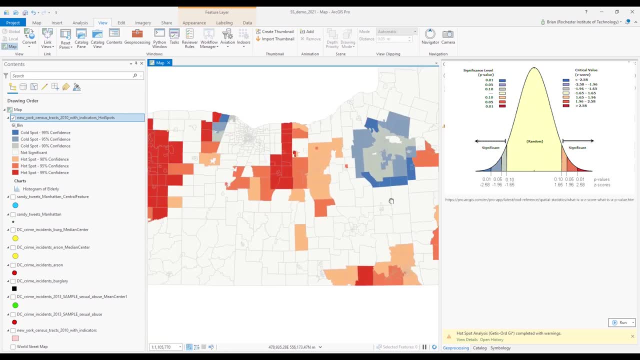 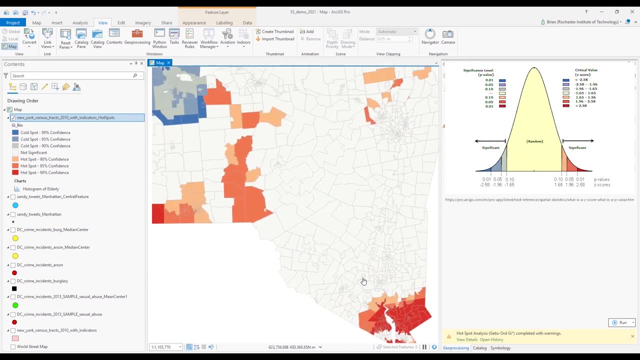 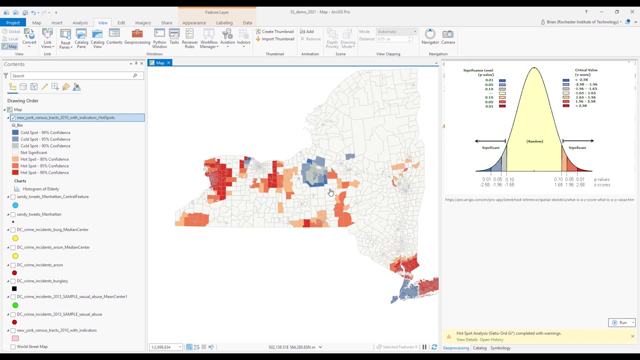 And there's actually a significant, A significantly insignificant amount or a cold spot over here and so forth, And if you examine the map you'll see these trends in different areas. So that concludes this very brief demonstration of some basic spatial statistics methods using. 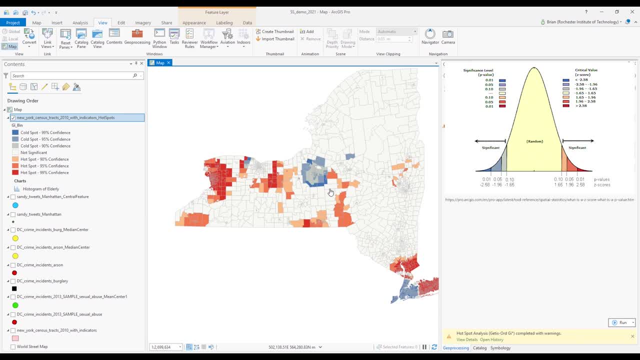 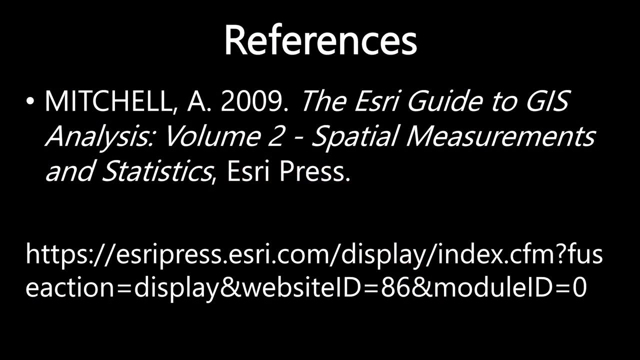 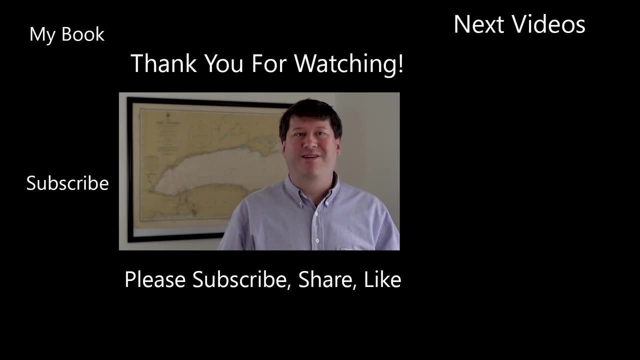 ArcGIS Pro software. Of course, this is a huge, massive topic and I encourage you to learn more about spatial statistics, as this is really just the beginning. The following are references used for this lecture: Hi, this is Brian Tomaszewski.